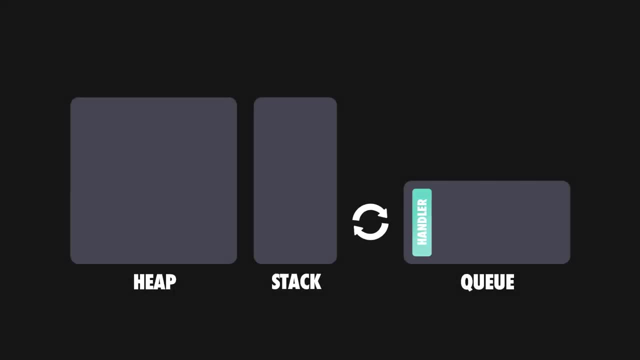 an associated event handler. The handler function will be pushed into the callback queue first. The event loop is always monitoring this queue. Whenever the stack is empty, tasks are moved from the queue to the stack and code is executed. Any object needed during this execution will be allocated in the heap. 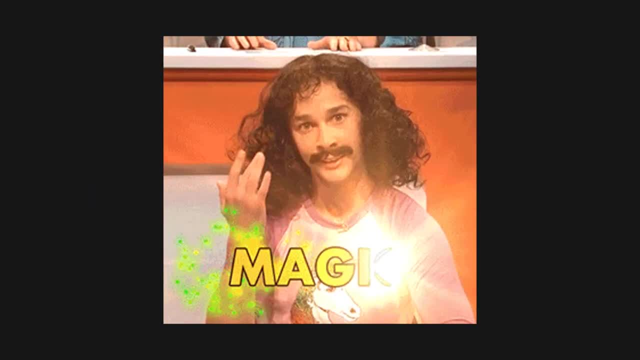 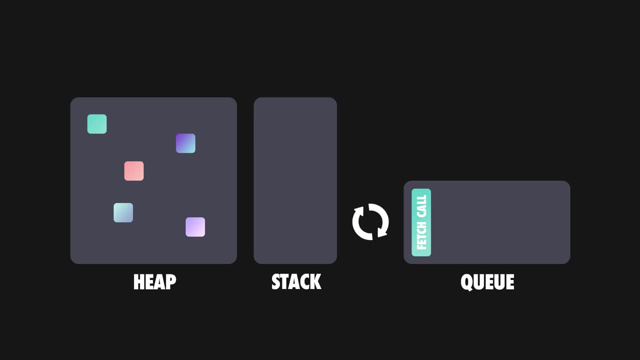 This async callback-based model is what allows your code to run smoothly, despite some long-running tasks like working with a network. In practice, whenever a call to the server is performed, the request is dispatched to the fetch API and the event loop clears the stack When the response is available. 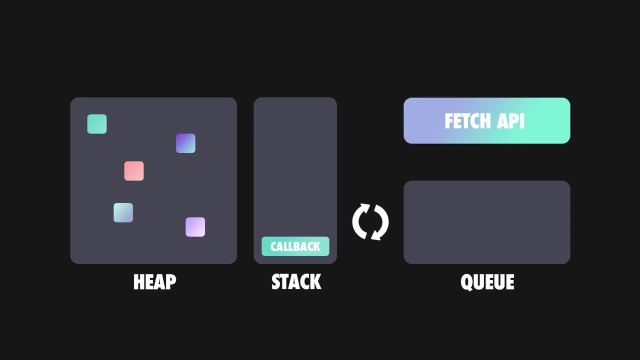 a callback is pushed in the queue and will end up being processed when its turn comes. Okay, so this model works, but you can still run into scenarios when the UI thread becomes blocked. Imagine, for instance, placing a function like this one on the stack. 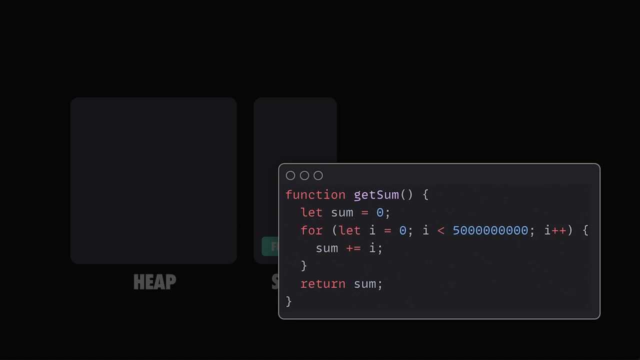 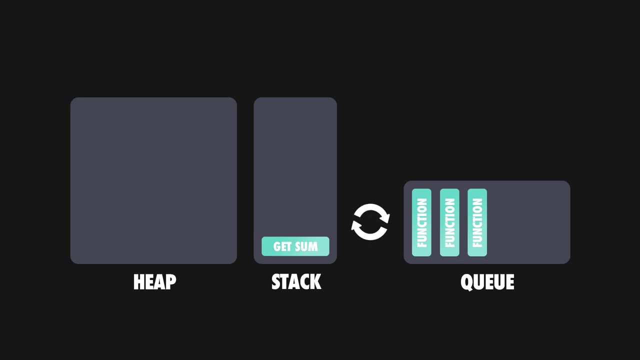 Calculating the sum will take a few seconds, even on powerful devices. While the for loop is executed, the function will stay on the stack and all other tasks will wait in the queue. Granted, it's not that often that you need to sum up billions of numbers. 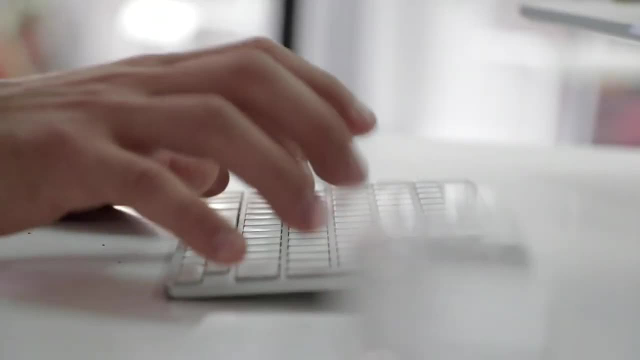 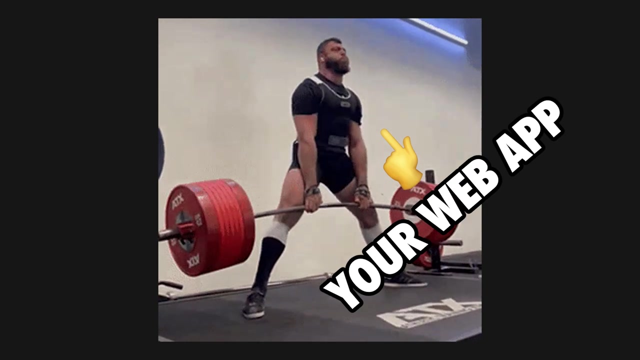 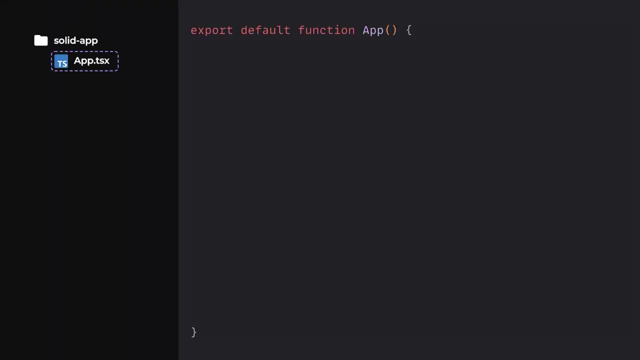 However, the reality of today is that modern front-end development interacts with AI libraries and complex WebAssembly algorithms, so handling heavy, intensive workloads might become a pretty common requirement in the near future. Next, let's look at some code. I defined a plain, solid component with two signal values. 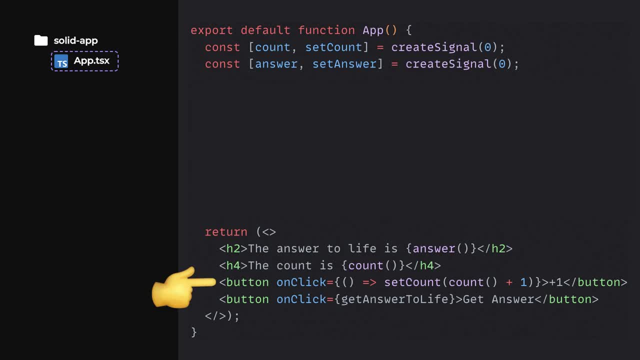 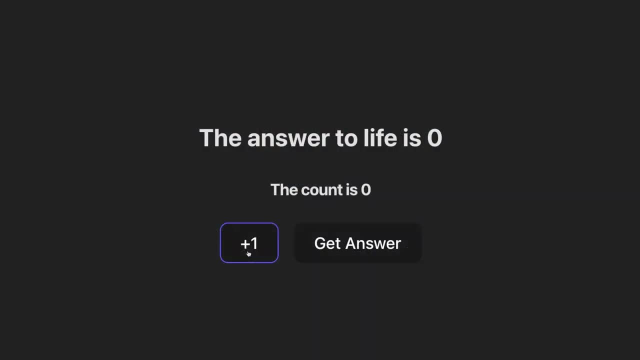 The counter value is simply incremented when the plus one button is clicked. The answer to life value will take a while to compute, however, due to the time-consuming for loop. At runtime we can seamlessly increase the counter, but once the getAnswer button is clicked, 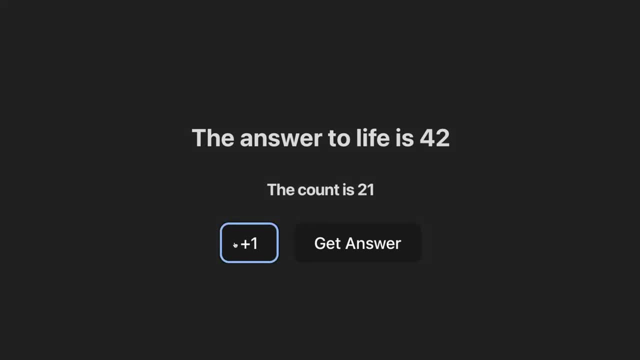 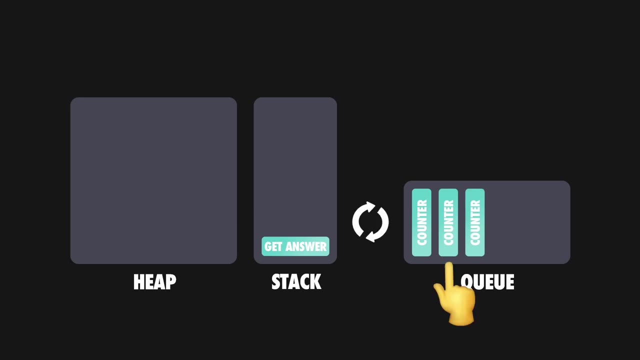 the UI will be non-responsive until the for loop is completed. Going back to the architecture diagram, whenever I'm clicking on the button to increase the counter, all callbacks will be pushed in the queue, but the event loop can't move them to the stack. 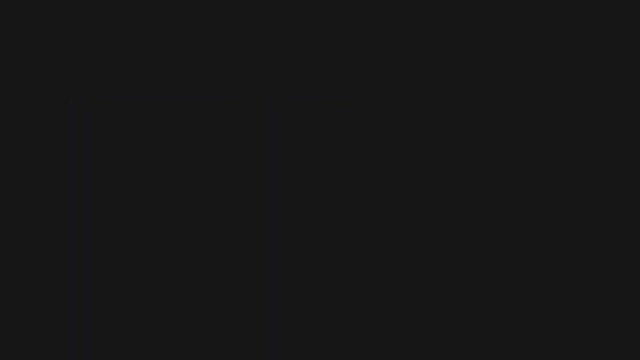 until the getAnswerToLife function finishes its execution. This is where web workers can help, since they run scripts in the background on separate threads. Compared to the UI thread, web workers have one big limitation: They can't interact with the DOM. 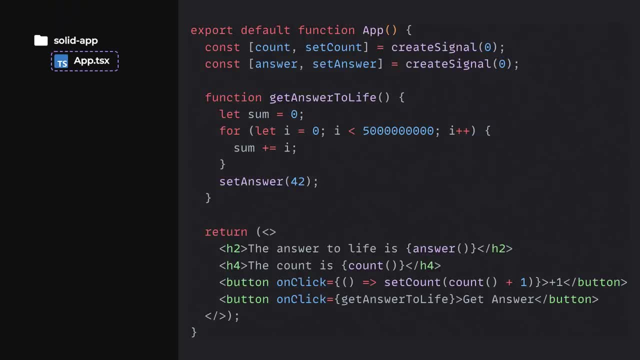 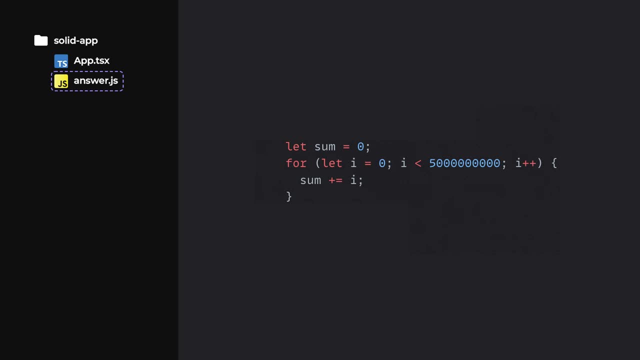 This makes using web workers very similar to the experience of working with the network. So let's move our long-running task into a new script called answerjs. The main thread and the worker will communicate with each other via messages. To accomplish this, we'll wrap our worker code in a non-message function.